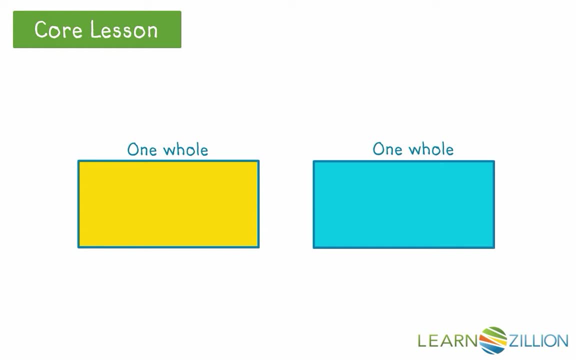 Here you can see what two different rectangles look like. I can partition one whole into three equal parts, with each region being called one third, by making two vertical lines or two lines going up and down to make three equal parts. Looking at the blue whole, I can also partition this one into three equal shares by drawing lines that are horizontal or left to right. So you'll notice I made two equal parts and I can also partition this one into three equal shares by drawing lines that are horizontal or left to right. So you'll notice I made two equal parts and I can also partition this one into three equal shares by drawing lines that are horizontal or left to right. So you'll notice I made two equal parts and I can also partition this one into three equal shares by drawing lines that are horizontal or left to right. So you'll notice I made two equal parts and I can also partition this one into three equal shares by drawing lines that are horizontal or left to right. So you'll notice I made two equal parts and I can also partition this one into three equal shares by drawing lines that are horizontal or left to right. So you'll notice I made two equal parts and I can also partition this one into three equal shares by drawing lines that are horizontal or left to right. 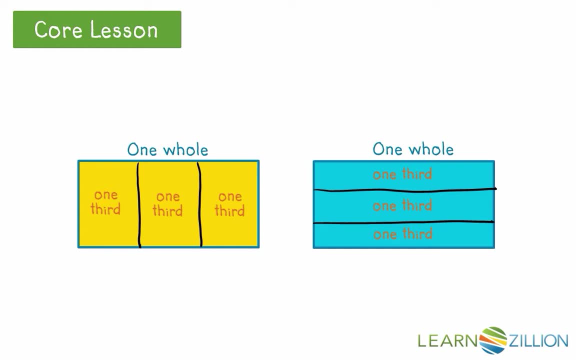 So you'll notice I made two equal parts and I can also partition this one into three equal shares by drawing lines that are horizontal or left to right equal parts, so each share is known as one-third of the whole. You will notice. 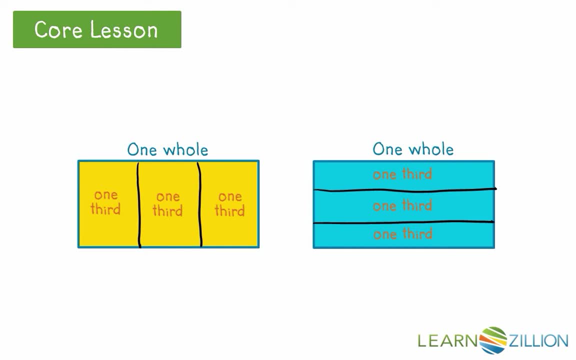 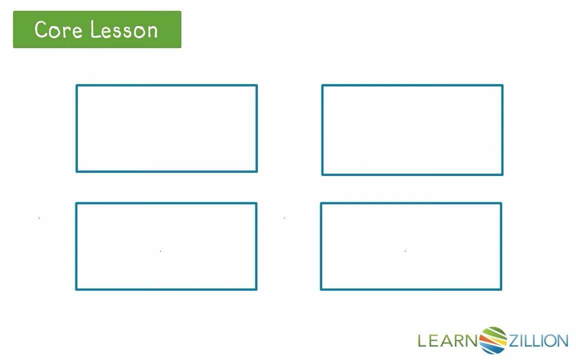 that the three shares in the yellow rectangle do not look the same as the three shares in the blue rectangle, but they each take up three regions of the whole they are inside of, so they are each one-third of the whole. Here you can see four different rectangles that are each one whole. I can partition one whole. 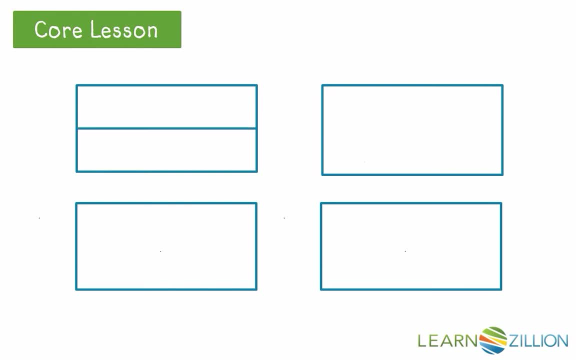 into four equal shares, with each region being called one-fourth, by partitioning the rectangle with a horizontal line or line that goes left and right, and make it into two equal shares. Then I split the two equal shares in half again to make four equal shares. So you can see that I now have four equal shares of. 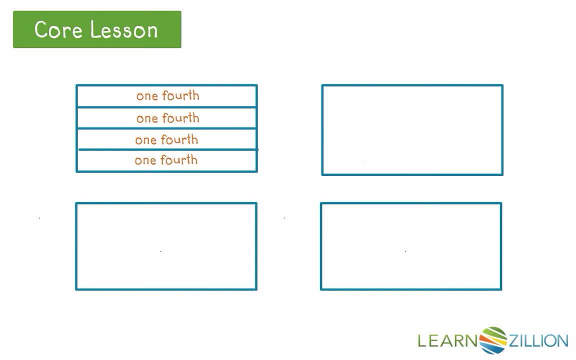 the whole, So each share is called one-fourth. I can also partition one whole into four equal shares by making a vertical line during them, down the middle, to make two equal parts. Now I will split each of those parts in half, again by two more vertical lines. Now I have four equal parts. so if I have four, 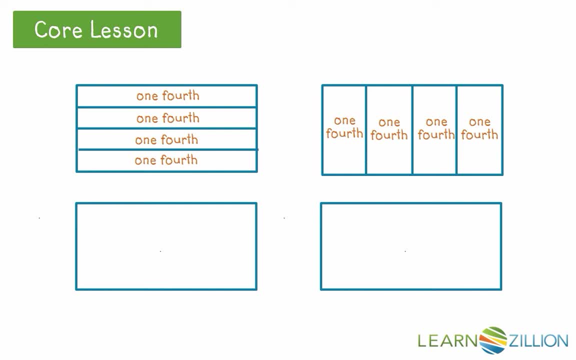 equal parts. each of those shares is one-fourth of the whole. Let's look at this bottom left whole. I can first partition this into two equal shares by making a vertical line during the middle. Now I am going to partition each of the two. 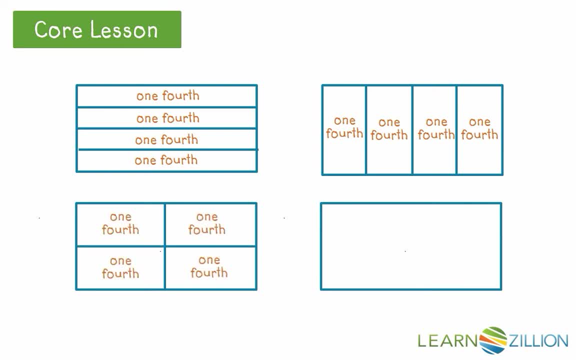 halves in half again with a horizontal line. Now I have four equal shares, with each region being called one-fourth of the whole. Sometimes my shares inside of the whole change their shape and look exactly the same as the other ones, But as long as they take up the same, 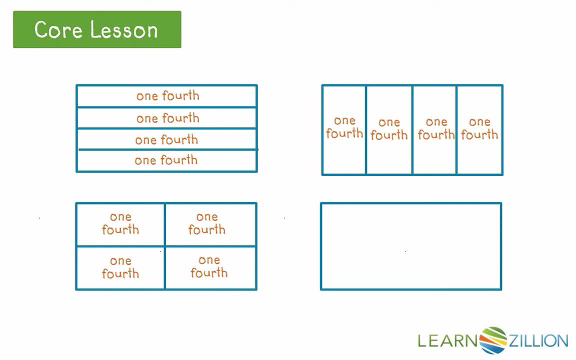 space as the other regions, they are a fraction of the whole. So let's take a look at that For this rectangle. I am going to first partition it down the middle into two equal parts. Then let's just look at the half on the left. I am going to partition that into two equal 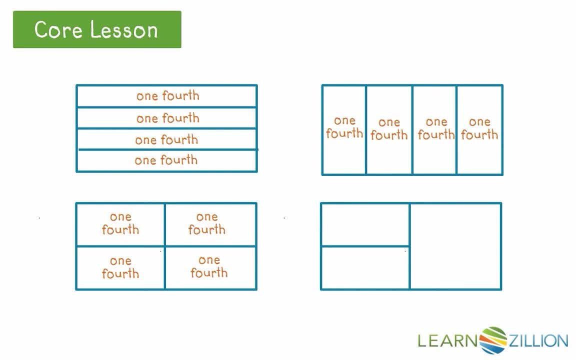 parts by making a horizontal line. Then if I look at my half on the left, I am going to partition that piece in half by making a vertical line. So I have now cut each of my halves in half So I know each of the pieces are equal to each other and I can say they are. 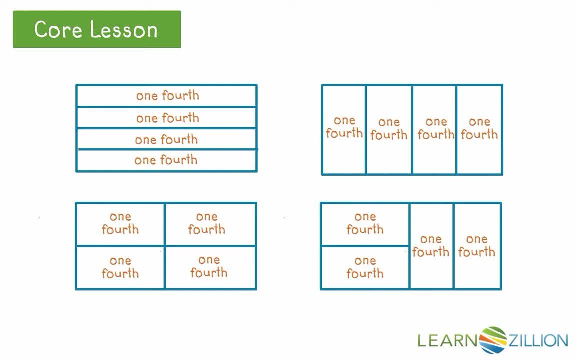 each one-fourth of the whole. So, if we are correct, each share in all of the rectangles should be the same, Because they are each one-fourth of the same whole, just cut in different ways. So let's look at this first rectangle and one of the fourths. I am going to cut this fourth in. 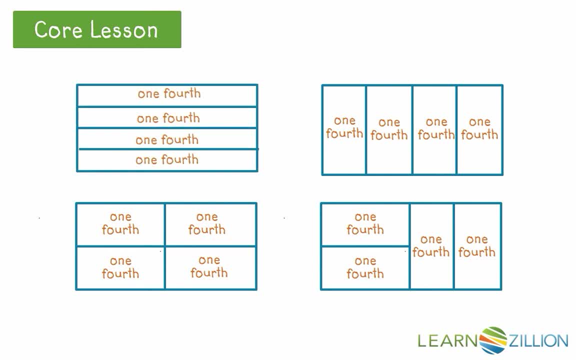 half to be able to move it around. So I have my half and my other half that make that one-fourth. Now you will notice that when I take each of these two halves and turn them vertically, I can place each of them on one-fourth in the top right rectangle and you notice they. 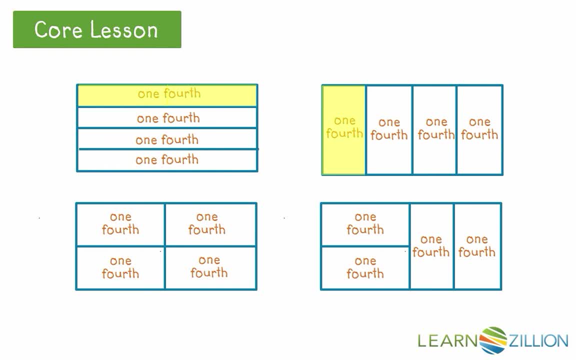 do indeed take the same amount of space as that one-fourth. Let's check this again. in the bottom left corner, These two pieces of the fourth should also fit on the one-fourth in the lower left rectangle. So I will put one, two, both pieces of my fourth on this. 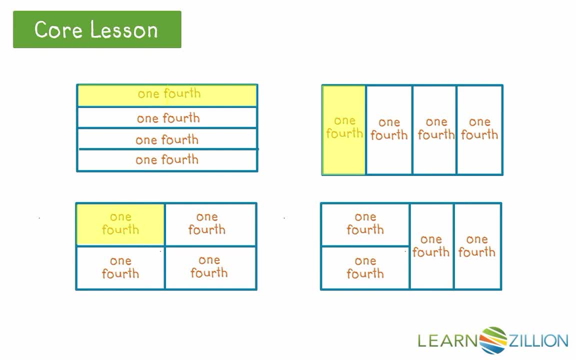 one And they also take up the same amount of space. So they are equal and both one-fourth. On this last rectangle, I can take those two pieces that are now vertical, place them inside this one-fourth or inside of this one-fourth, and it also takes up the same amount of space. 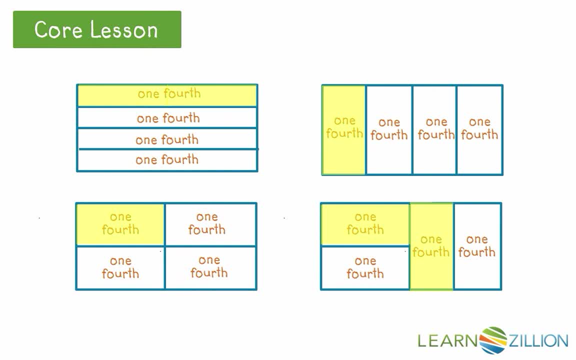 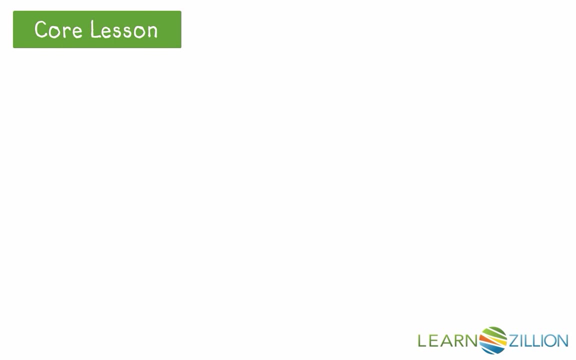 as the piece. So you will notice that even though the fourths look different, they are all one-fourth and the same size because they are inside of the same size whole that was partitioned into four equal parts, just different ways. It is important to note it that when 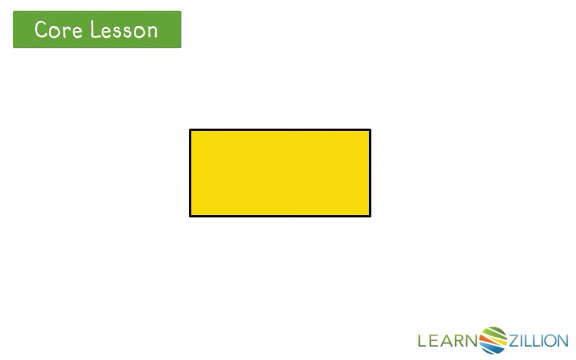 partitioning rectangles into same size shares. they are equal to each other and take up the same amount of space. So you can see I have one whole and I have partitioned it into four equal shares Where each region is one-fourth of the whole. 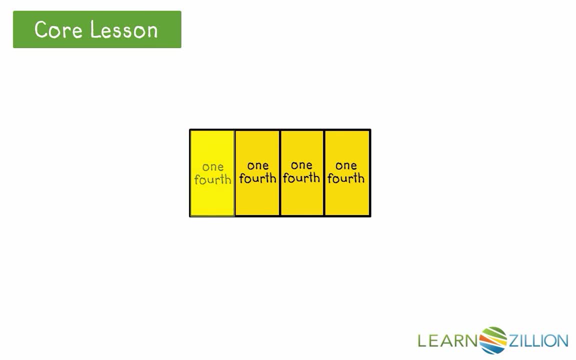 So you can see I have one whole and I have partitioned it into four equal shares where each region is one-fourth of the whole. I am going to highlight each share so we can see if the four shares are in fact equal. So one-fourth is yellow, one-fourth is green, one-fourth is blue and one-fourth red. 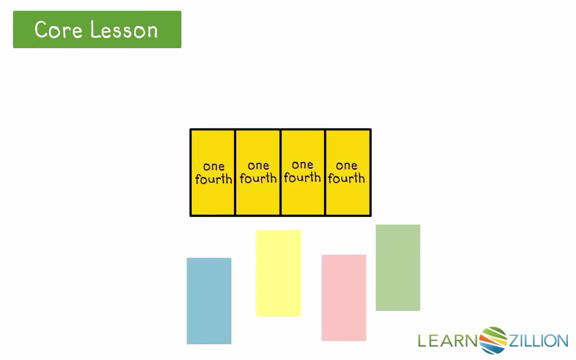 Now that I have a copy of each of the fourths, I will pull it away from the whole. If I line up my four shares, since they are supposed to be equal, they should all line up on top of each other. Let's try it out. 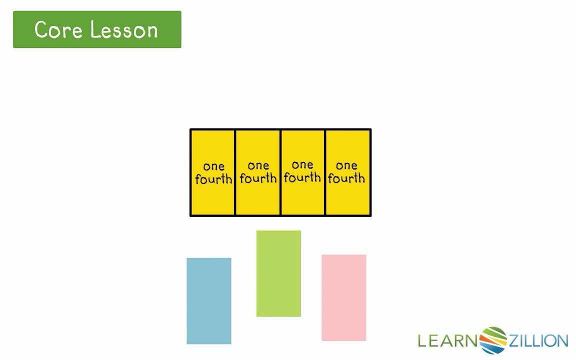 I have one-fourth yellow here and I will place one-fourth green on top of it to show that they are the same size. Now I have my one-fourth green and I can put it on top of my other fourths and you can. 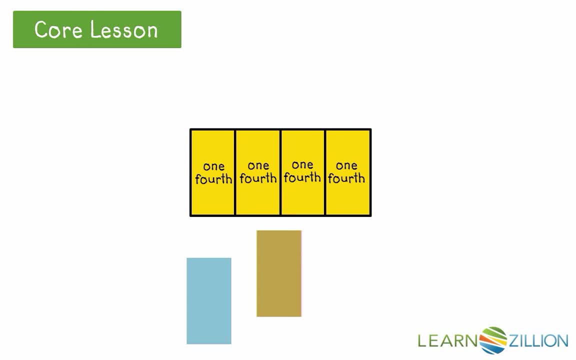 see it fits on top of it, so they are equal. Now I will also put my blue on top of the other fourths and you can see it also takes up the same amount of space. it is the same size. So you can see the shares of a fraction.